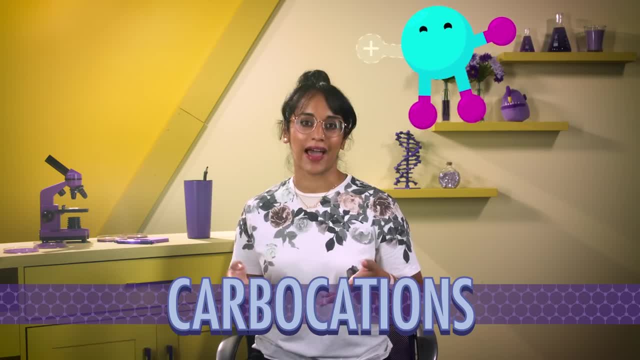 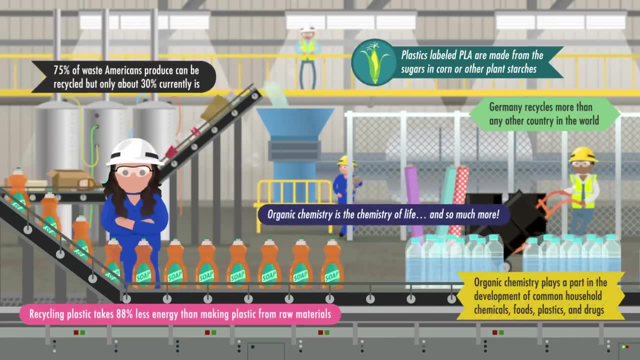 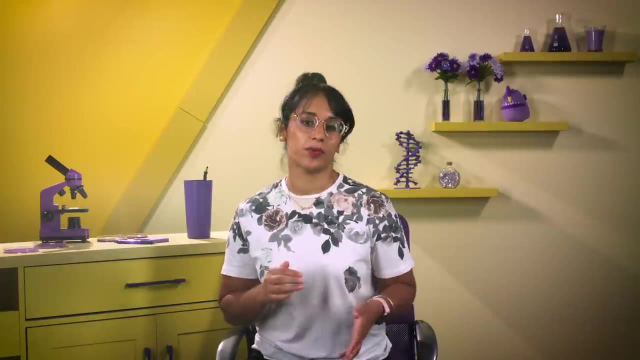 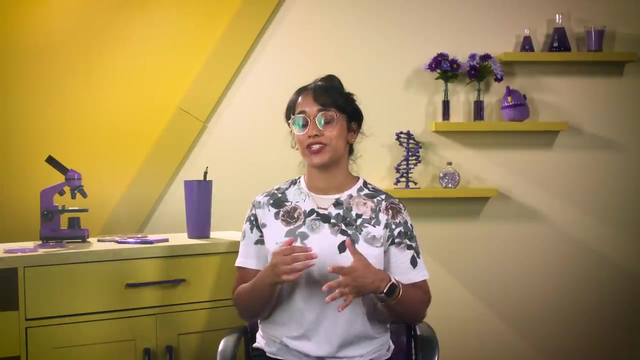 carbocations, those molecules with positively charged carbon atoms. An alkene is a molecule containing carbon-carbon double bonds. Unlike single bonds, double bonds are rigid. They can't easily rotate because the pi bond would need to break first, and that costs energy. 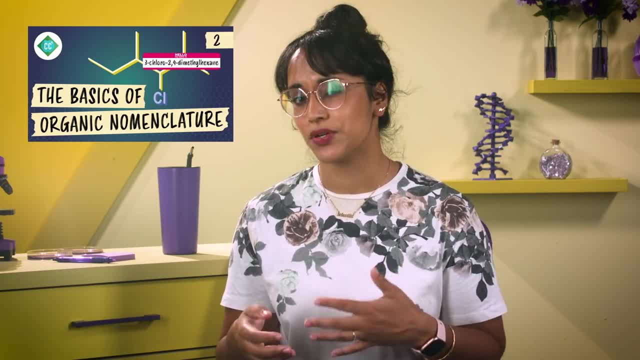 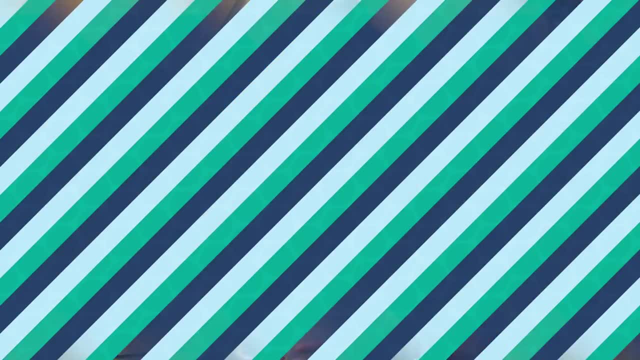 In episode 2, we talked briefly about cis and trans isomers of alkenes. As a refresher. this naming system helps us describe two different geometric isomers around a double bond. For example, let's look at pentuene. 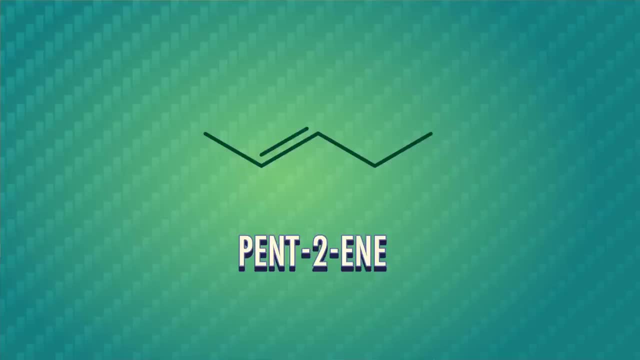 If the methyl and ethyl groups are on opposite sides around the double bond, we call it transpentuene, And if the methyl and ethyl groups are on the same side around the double bond, we call it cispentuene. 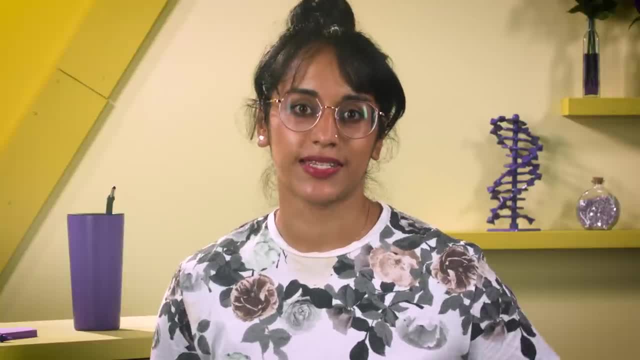 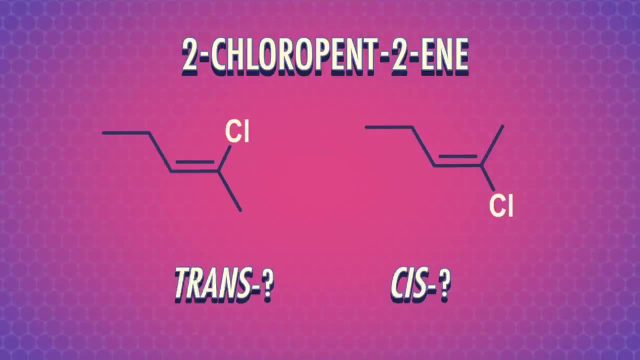 But in the context of alkenes, cis and trans is an old-school naming system that only works when the double bond carbons are attached to two hydrogens and two R groups. If we consider something like 2-chloropentuene, 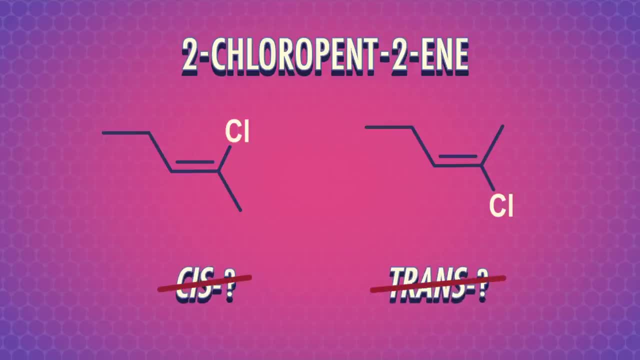 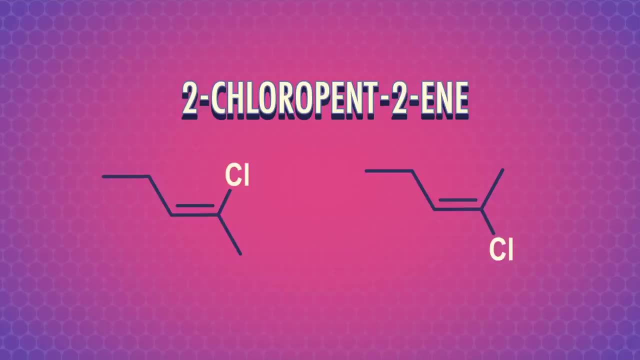 the cis and trans system fails to help us accurately communicate where the groups are, so we need a better way. Thankfully, organic chemists have us covered. Similar to assigning R and S enantiomers of molecules, we can prioritize the groups on each carbon of the double bond. 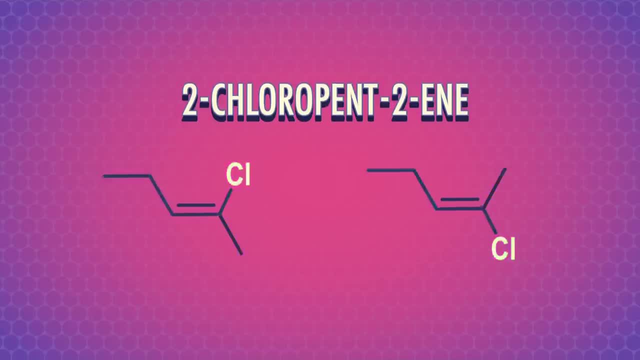 using the rule that higher atomic number means higher priority. In this first isomer of 2-chloropentuene, the carbon on the double bond is called a trans. The carbon on the left side of the double bond is attached to an ethyl group and a hydrogen atom. 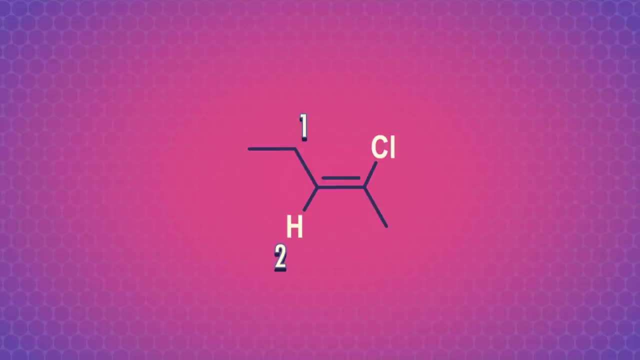 The ethyl wins priority because its carbon has a higher atomic number than hydrogen. The carbon on the right side of the double bond is attached to a chlorine and a methyl group. Here the chlorine wins priority. If we mark our priority, winners and losers. 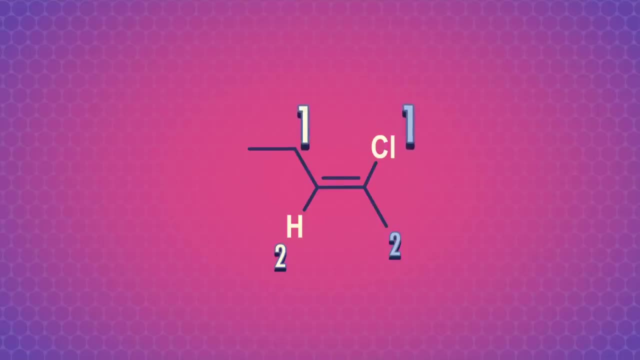 we can see that high-priority groups on each double-bonded carbon are on the same side of the double bond. So this is the Z-isomer, which comes from the German word Zusamen for together. So we have Z-2-chloropentuene. 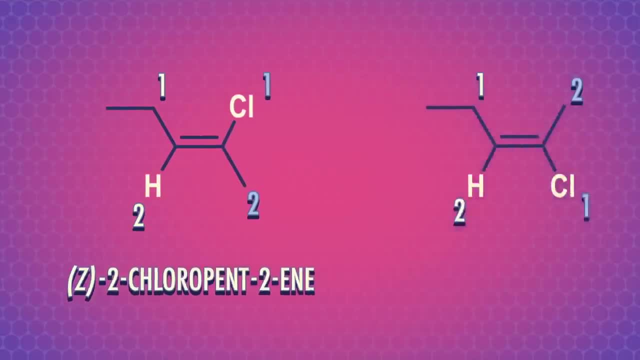 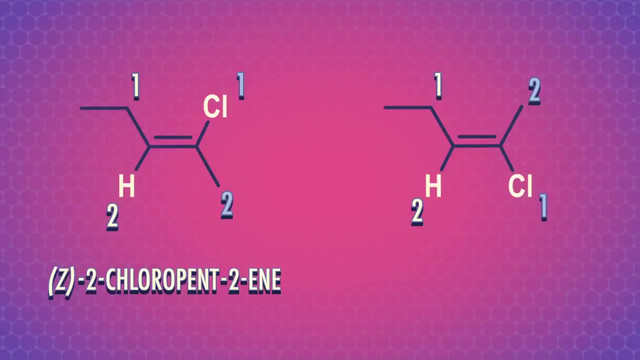 The other isomer of 2-chloropentuene has high-priority groups on opposite sides with respect to the double-bonded carbon atoms. So this is the E-isomer, derived from the German word entgegen, or opposite. 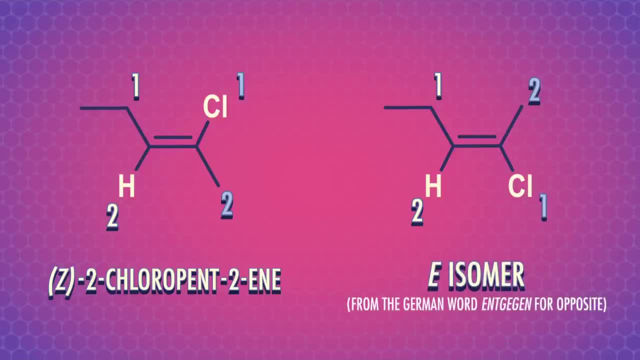 I don't have quite a clever way to remember this, but I remember it as E-cross for across, So it's E-2-chloropentuene. Assigning priorities isn't always so easy, so if we have a tie we need to keep hopping along. 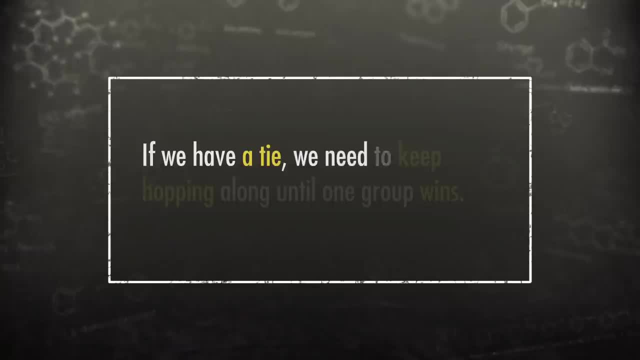 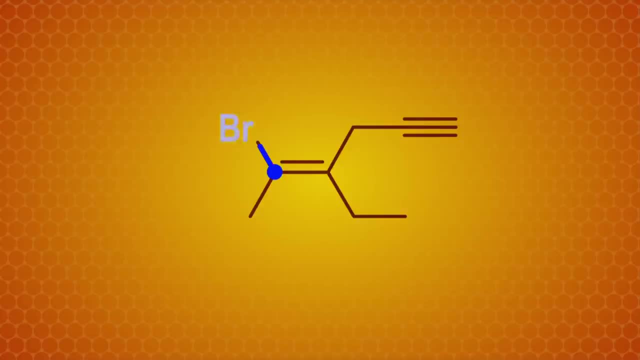 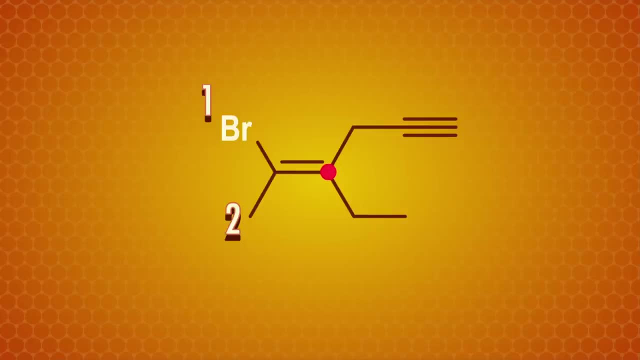 Bromine wins priority over the methyl group. But on the right-hand carbon, the first position gives us the same thing – a carbon with two hydrogens attached, A tie. So we have to keep going and compare the next two atoms. There we can see that the triple-bonded carbon wins priority because it's like three carbons at once compared to one carbon on the other side. 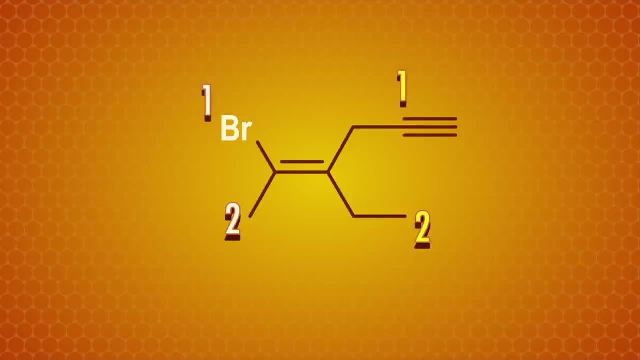 Now we can see our priority winners are on the left-hand side. Now we can see our priority winners are on the same side. so it's a Z-isomer and we call this guy Z-5-bromo-4-ethylhex-4-N-1-Ine. 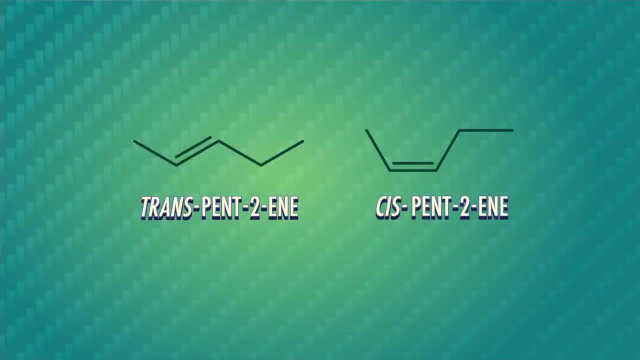 Now we can see our priority winners are on the left-hand side. so it's a Z-isomer and we call this guy Z-5-bromo-4-ethylhex-4-N-1-Ine. Returning to our first example, transpentuine can be more precisely called epentuine, and the cis-isomer is the Z-alkene. 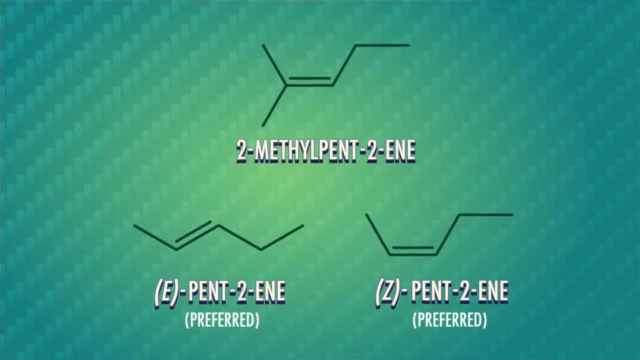 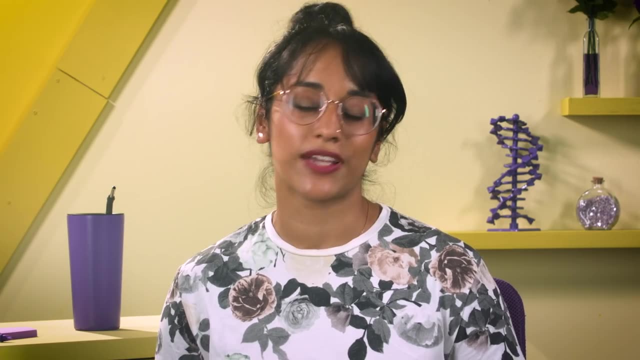 And if one side of the alkene has two of the same group, like 2-methylpentuine, here we don't need to use E and Z. So now we know how to name alkenes a little bit better and we can start playing around with some reaction chemistry. 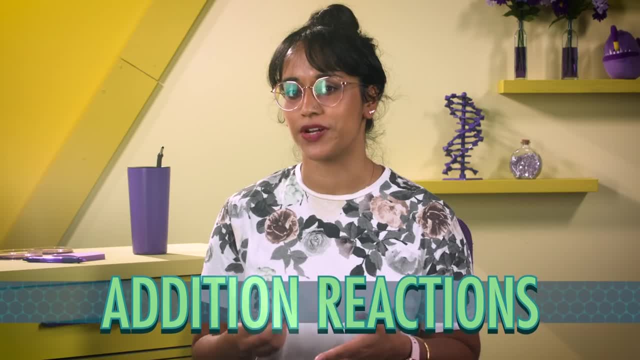 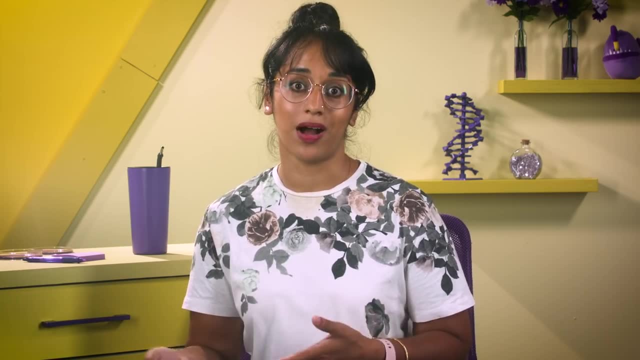 Many of the chemical reactions associated with alkenes are addition reactions, which means the pi electrons are attracted to electrophiles and groups get added to the carbons on each side of the double bond. In episode 12, we saw what happens when we mix hydrogen bromide and cis-butylene. 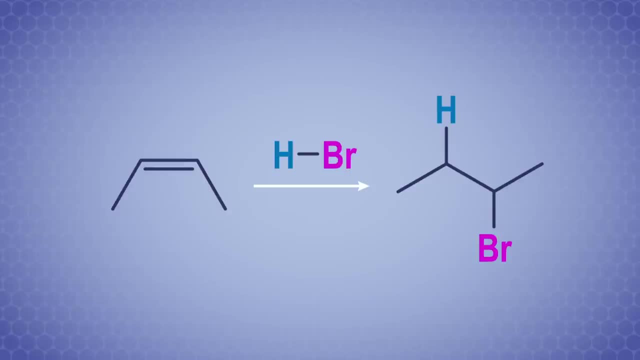 It's a pretty straightforward nucleophilic attack where the alkene double bond attacks a proton and one of the previously double-bonded carbons gets a bromine. No matter which carbon bonds to the bromine, the product is the same. 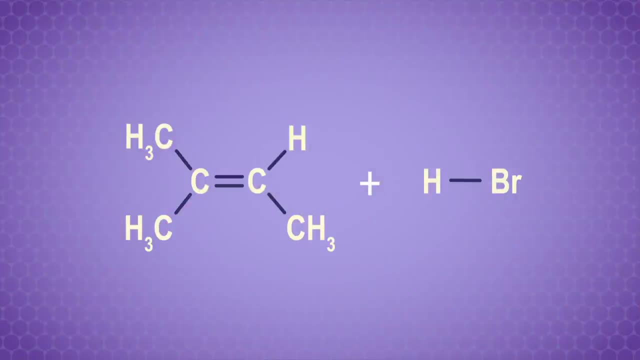 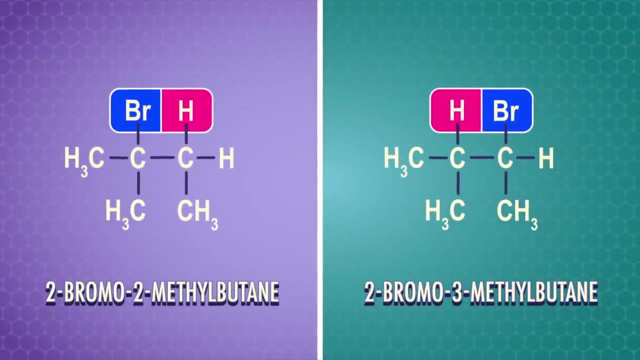 But things aren't usually so simple. For instance, if we add hydrogen bromide to 2-methylbutylene, which isn't symmetrical, we can potentially make two different products. Here's the catch, though: When we do this reaction in a lab, we only make one of those two products. 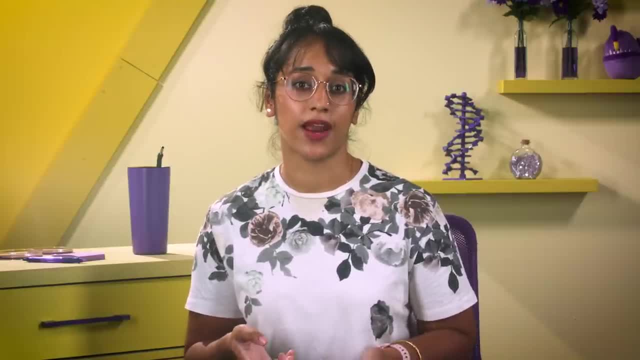 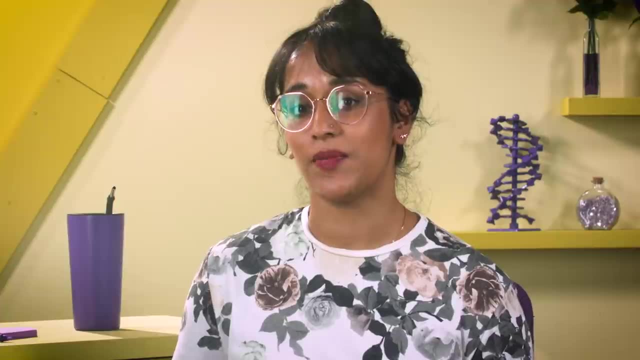 This seemingly mysterious observation actually has a pretty good explanation. It's because of the stability of different carbocations which are positively charged carbon atoms. To see where carbocations come in, we have to break this reaction into steps. Remember that hydrogen bromide is a strong acid. 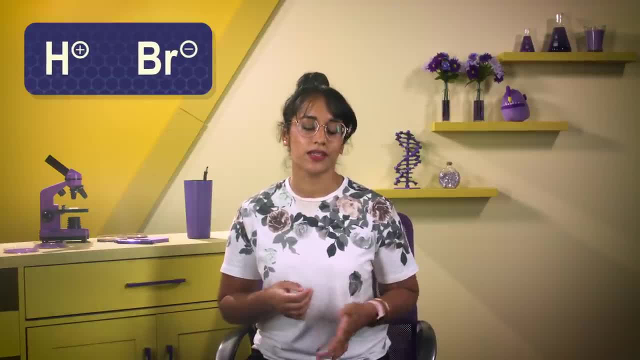 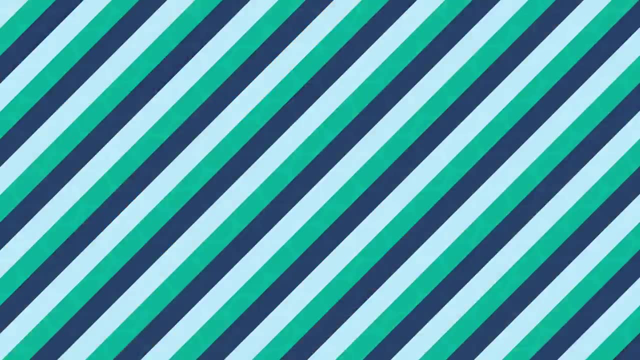 so it's fully dissociated from the carbons. It's dissociated into H-plus and Br-minus ions. Most textbooks show an attack on an undissociated molecule of hydrogen bromide, so that's how we'll show it in this series. 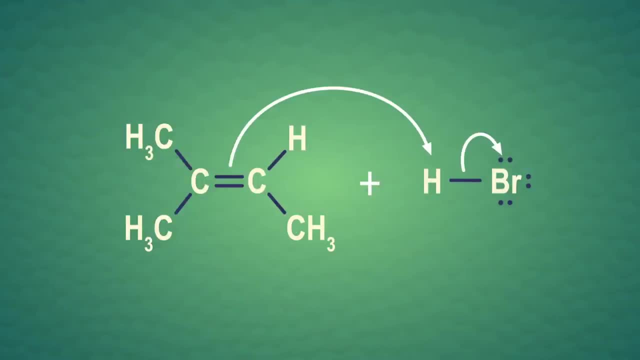 So first, the alkene initiates a nucleophilic attack on the proton formed by the dissociation of hydrogen bromide, donating a pair of electrons, snagging the proton and leaving the remaining carbon of the double bond short two electrons. This creates a positive charge, a carbocation. 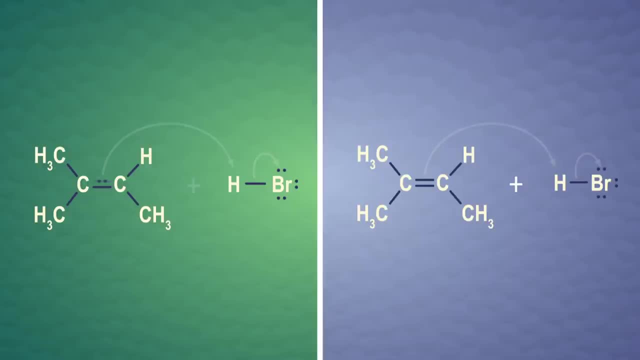 There are two possible carbocations that can form here: One where the positive charge ends up on a carbon surrounded by three other carbons, called a tertiary carbocation, And one where the positive charge is on a carbon surrounded by two carbons in hydrogen, called a secondary carbocation. 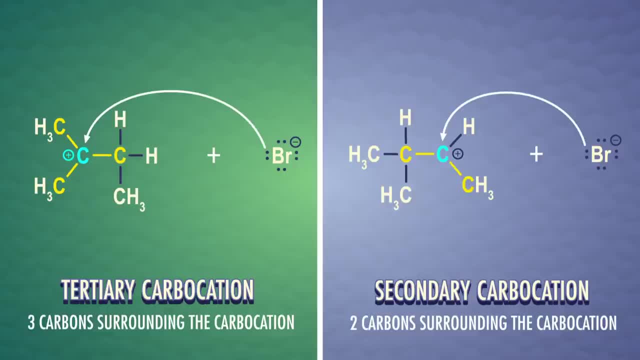 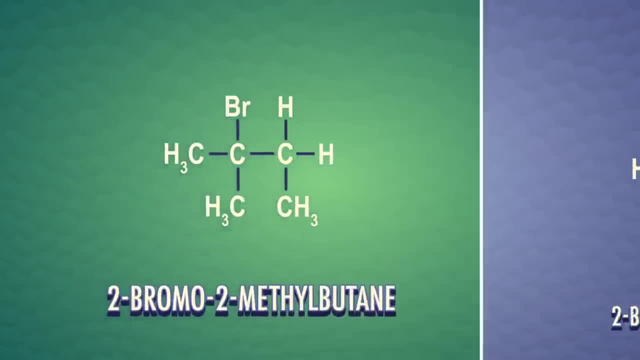 The next step is to form the product: a bromide, nucleophilic attack on the carbocation to form a bond Where the carbocation forms ultimately determines what product we get And for some reason, the tertiary carbocation is what forms, because that's what leads to our observed product. So I don't know about you, but I'm wondering… why does this reaction happen this way? Well, we describe carbons with more carbon-carbon bonds as more substituted and more stable If we were to draw four similar carbocations as we replace carbon-carbon bonds with carbon-hydrogen bonds. 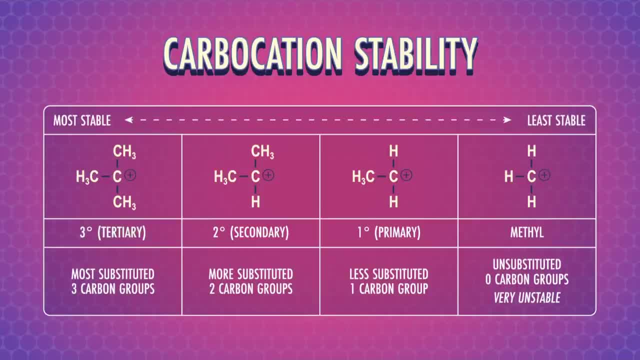 the carbocation becomes less and less stable. In other words, a tertiary carbocation is more stable than a secondary one, which is more stable than a primary one, which is more stable than a platelet-methyl carbon, which is more stable than a tertiary carbocation which is more stable than a primary one, which is more stable than a spin of aibel, which is more stable than a methyl carbon. If you see the carbon right, cons妹, you'll notice that course gets lead into the Martian react of carbos and just that's it. 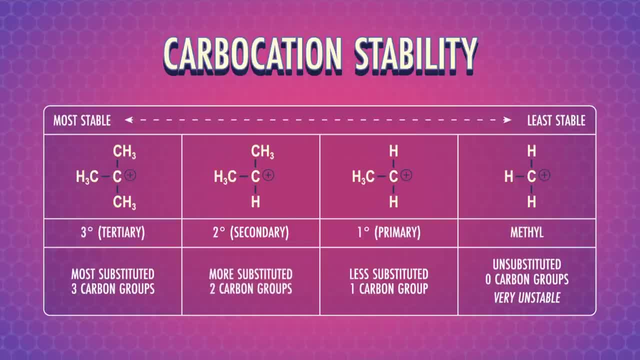 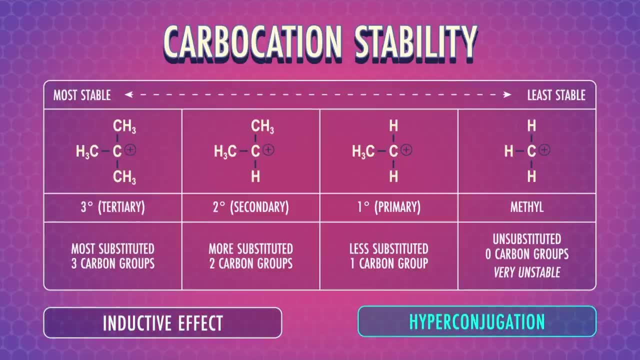 carbocation. The more substituted carbocation is stabler than a less substituted one. This pattern instability is caused by two things: an inductive effect and hyperconjugation. The inductive effect is where the electron density is sort of spread out through the sigma bonds to stabilize the positive charge. It's like if you're trying to balance on a unicycle. The carbon-carbon bonds are your friends. with their feet firmly on the ground, who can stick out a hand or some electrons and bonds for support? 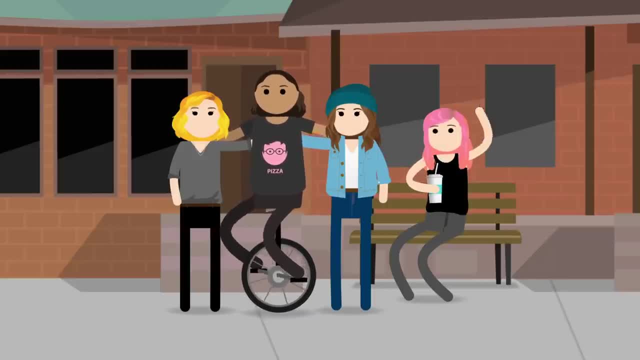 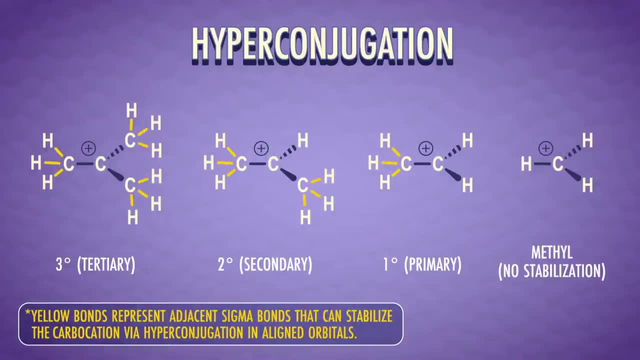 However, the carbon-hydrogen bonds are friends that aren't strong enough to help. Basically, more alkyl groups surrounding the carbocation lead to a bigger stabilizing effect. Hyperconjugation is an even more spread-out kind of stabilization borrowing electron. density from sigma bonds, kind of sideways from the positive charge, To sort of continue the unicycle metaphor. it's like instead of just a hand your friends actually lean their body up against it, Sort of like a big bear hug. So here too, additional carbon atoms have more sigma bonds that can stabilize the carbocation. 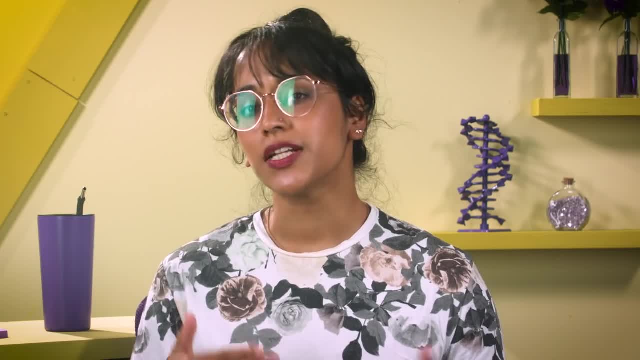 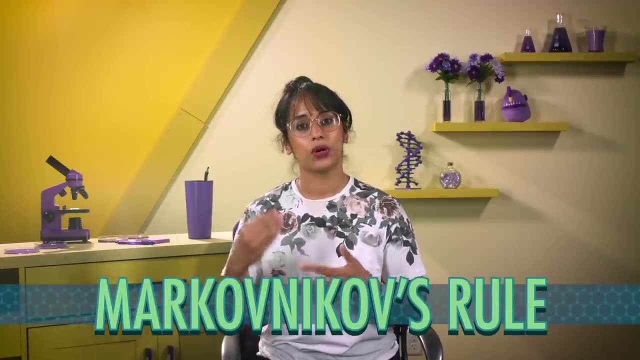 So when you add a hydrogen halide to an alkene, the product will be formed from the most stable carbocation. This pattern is called Markovnikov's rule. In these reactions the proton will add to the side of the double bond that has the most. 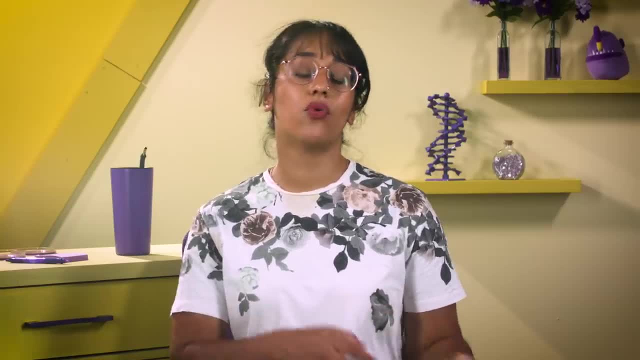 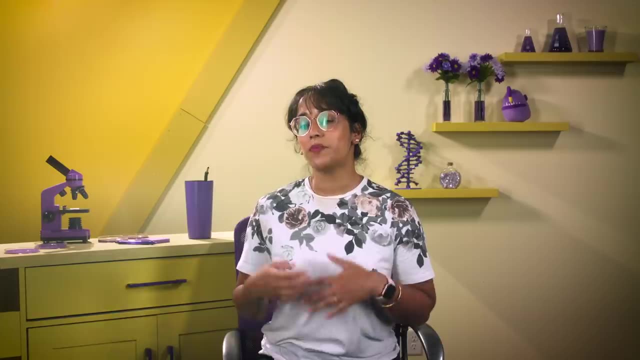 hydrogens. That means the positively charged carbon will be connected to more sp3 carbons, which means it's more substituted and therefore the more stable of the two possible carbocations. With practice we can use Markovnikov's rule to help us predict lots of products. 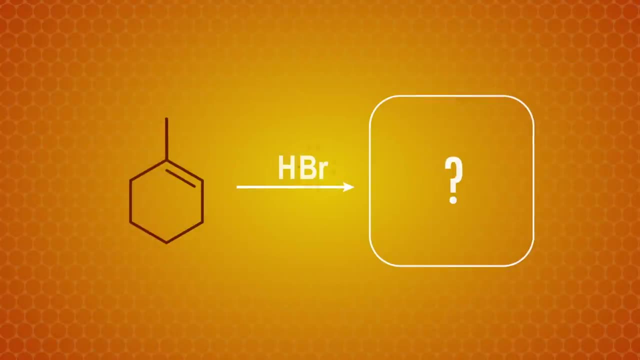 For example, let's try adding hydrogen bromide to 1-methylcyclohex-1-ene. We know the nucleophilic attack starts at the double bond and attacks the proton. Then, to follow Markovnikov's rule, we have to put the proton on the side of the double. 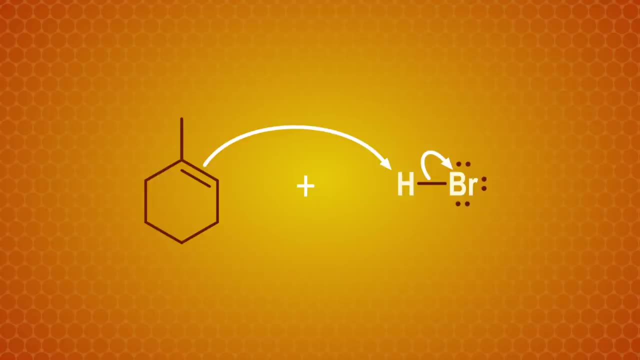 bond with the most hydrogens – that's the carbon. with one carbon-hydrogen bond instead of none, The positive charge will end up on the other side of the double bond, which is the carbon-hydrogen bond. If we add another carbon, which gives it more stabilization, we'll make a tertiary. 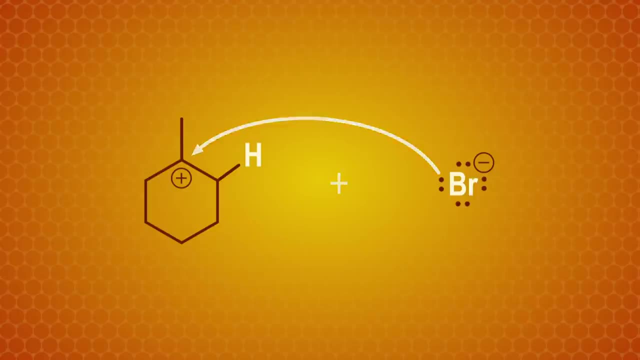 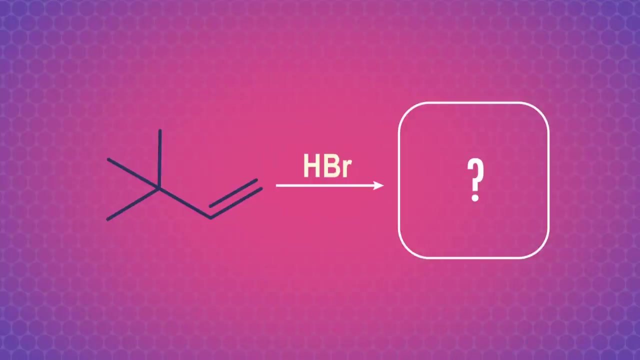 carbocation instead of a secondary one. The bromide does a nucleophilic attack And our product is 1-bromo-1-methylcyclohexane. Seems pretty simple, right, Almost too simple. So let's try another example and use Markovnikov's rule again to predict the product. 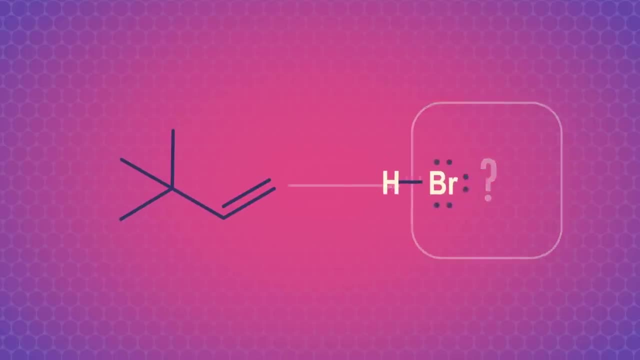 Here we have hydrogen bromide and 3,3-dimethylbut-1-ene. If we go through the same steps, do a nucleophilic attack? put the proton on the side of the carbon, with two carbon-hydrogen bonds instead of one, and get a positive charge on the other. 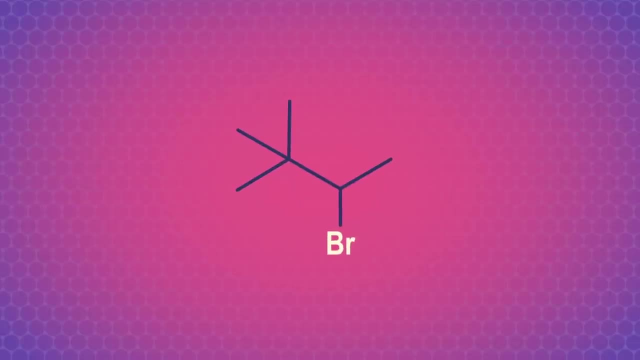 carbon, Our expected product would be 2-bromo-3,3-dimethylbutane. But when we do this reaction in the lab, we get a mixture of two products And our expected product is just the minor one, not even the majority. 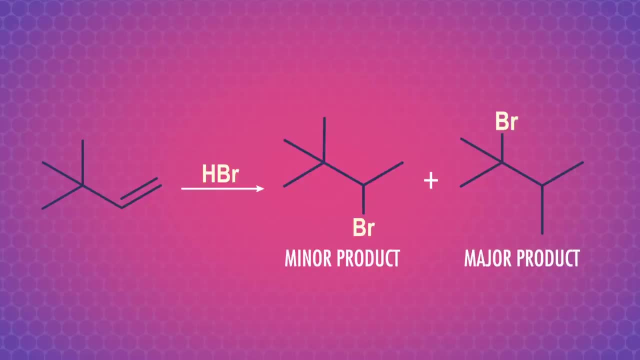 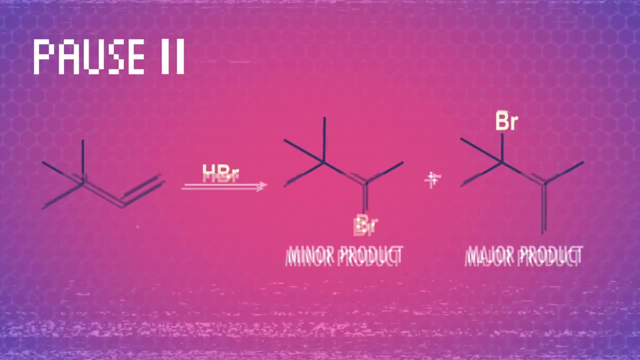 We just learned Markovnikov's rule, and now this reaction puts the bromine in a place where we didn't even have a double bond to start. Okay, Deep breath, Organic chemistry is tricky, but it does make sense with lots of practice. 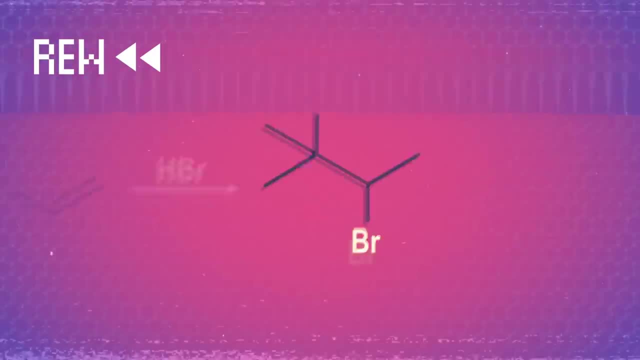 Are we really breaking science or is there something more subtle going on here? Let's see where and why this reaction gets weird. First, like we've seen before, the alkene attacks the proton from hydrogen bromide And the positive charge ends up on the carbon that creates the more stable secondary carbocation. 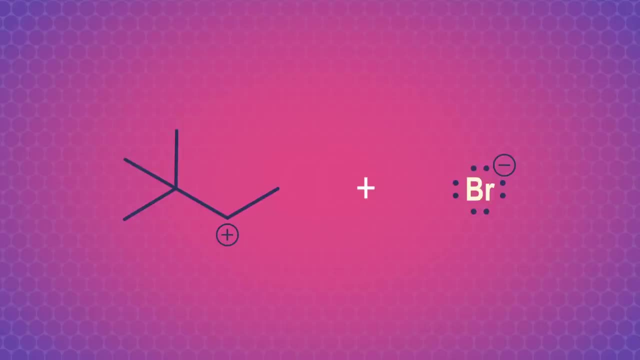 instead of the less stable primary carbocation that we didn't make. This is where I tried to do the next step of the reaction And how we got our minor product. But for the major product to form, the positive charge ends up on a different carbon somehow. 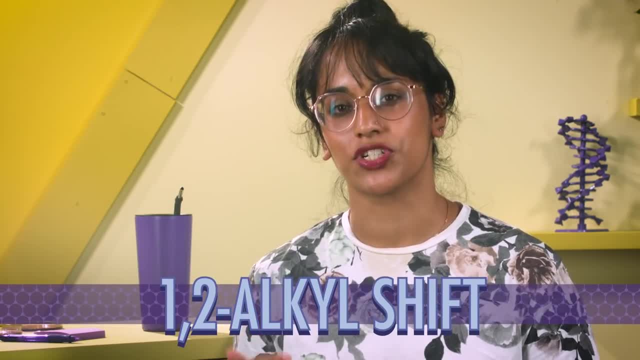 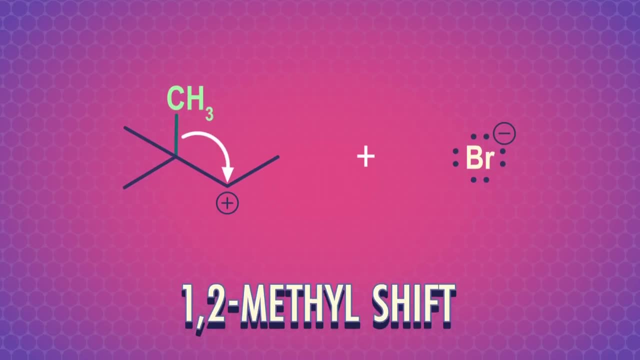 That somehow is a sneaky move called a 1,2-alkyl shift. As a reminder, alkyl groups are methyls, ethyls and things like that, And in this case it's a 1,2-methyl shift, where a methyl group- CH3, moves over to the 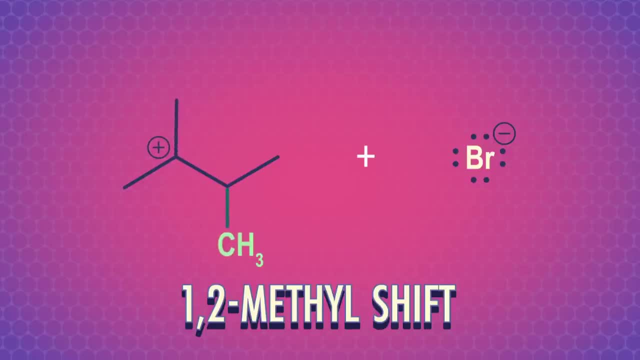 positively charged carbon next door, taking its electrons with it. This move only happens with groups on the adjacent carbon alkyl group And that's how we got our minor product. but for the major product to form, the positive charge ends up on the adjacent carbon atom. 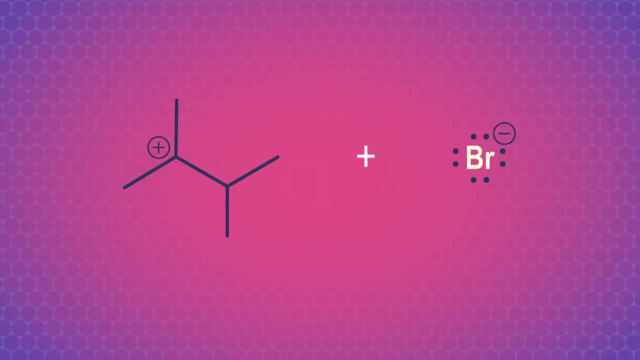 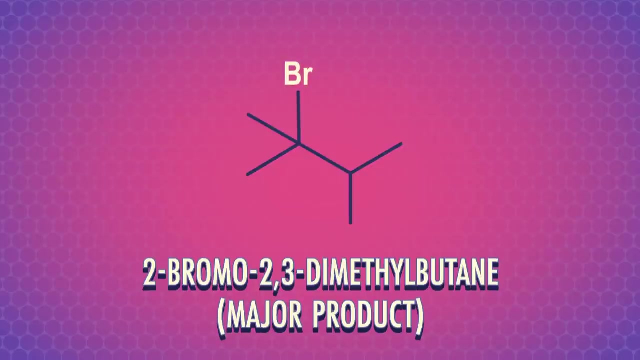 That creates a new, even more stable tertiary carbocation. So when the bromide does its nucleophilic attack, we get the major product that we see experimentally – 2-bromo-2,3-dimethylbutane. So technically, my earlier prediction wasn't wrong, it was just incomplete. 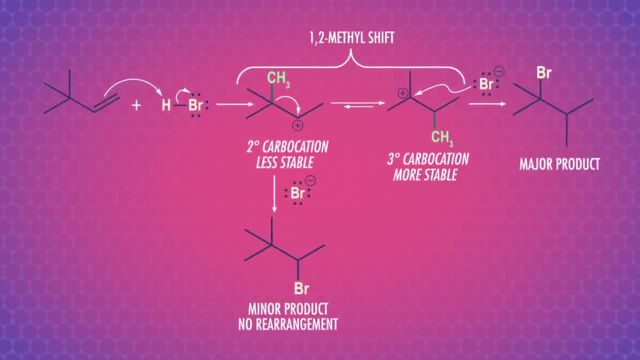 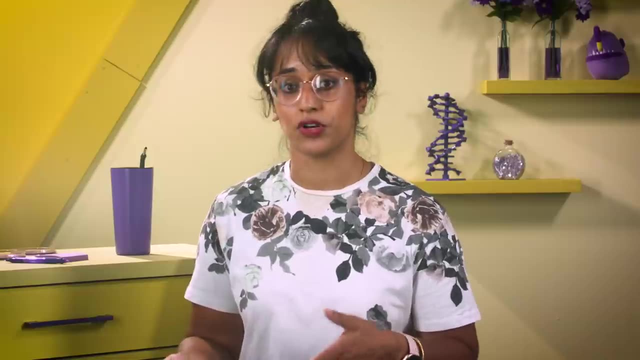 Depending on how we follow our reaction mechanism roadmap and whether the 1,2-methyl shift happens, this reaction can have two different products. Not all carbocations rearrange like this We saw with the first two reactions. This multidimensional map only happens when there's an even more stable carbocation. 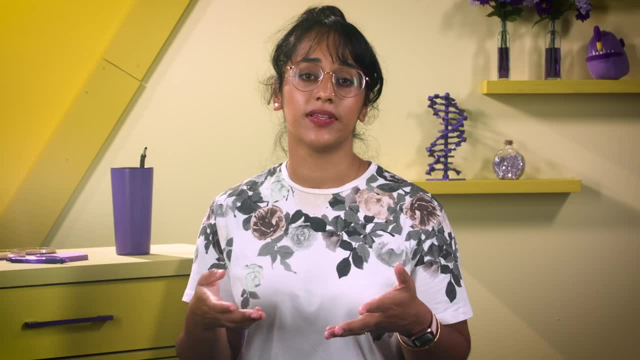 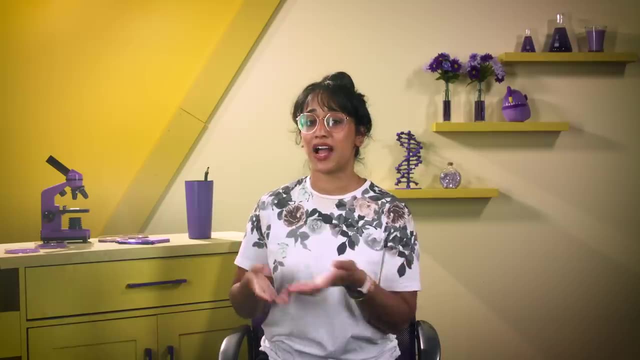 that can form. So we have to keep an eye out for carbons branching out next to the spot where the carbocation forms, And not just for shifty alkyl groups Turns out. hydrogen atoms can also do their own sneaky move, called a 1,2-hydride shift. 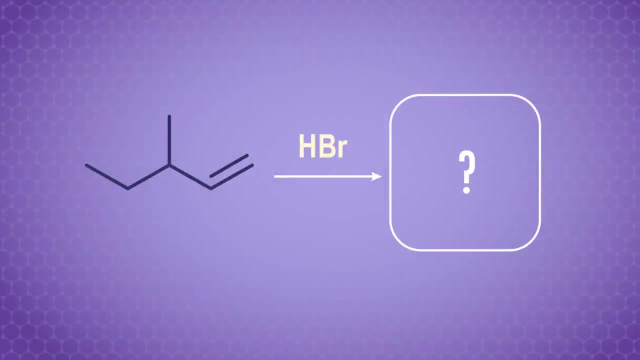 To see this in action, let's look at an example of hydrogen bromide and 3-methylpent-1-ene. We do the same nucleophilic attack initiated by our alkene and pick the second nucleophilic secondary carbocation as our product because it's more stable than the primary option. 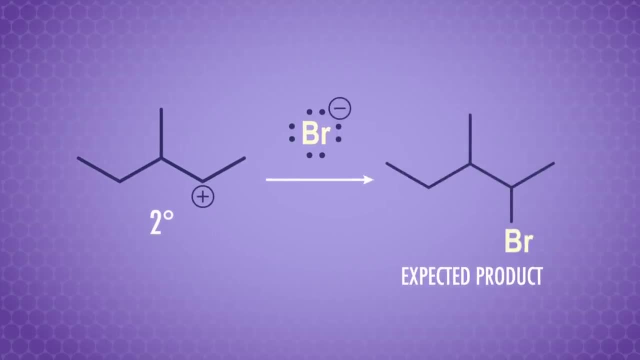 Then a reaction with the bromide would form the product 2-bromo-3-methylpentane. But this time we won't be fooled. We're keeping an eye out for more stable carbocations and what do you know? there's. 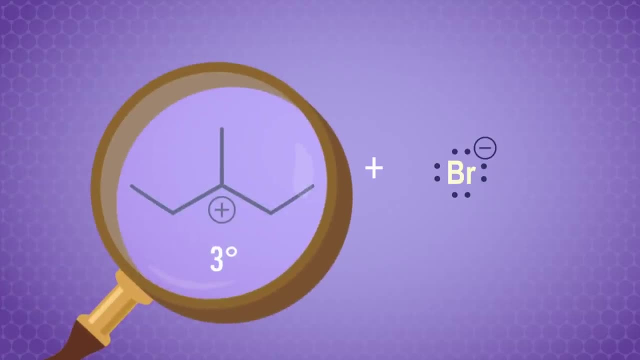 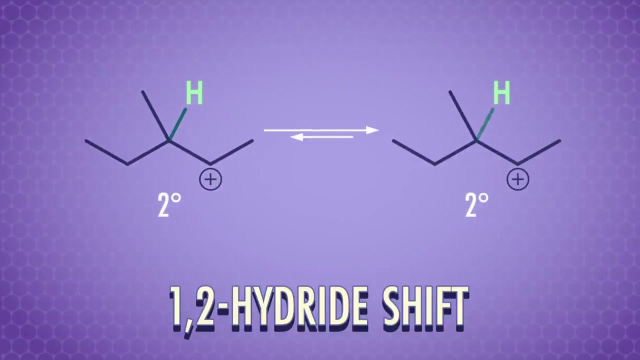 another possible product. Bumping the positive charge left 1-carbon would give us a more stable tertiary carbocation and we can make that shift happen with a 1,2-hydride shift. It's a very similar dance Where a hydride or hydrogen with its pair of electrons is a 1,2-hydride shift. 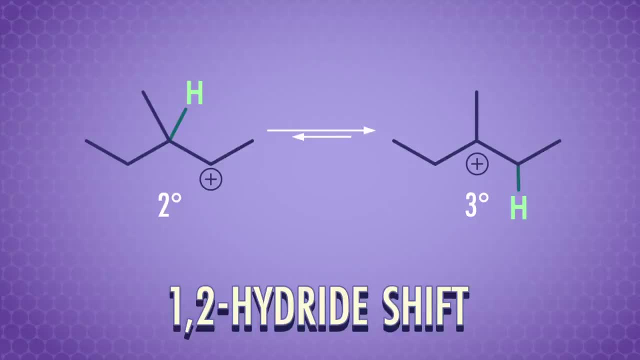 So we can make that shift happen with a 1,2-hydride shift. The hydrogen with its pair of electrons shifts over to the positively charged carbon next door By taking the electrons from its bond with it, the hydrogen leaves behind a positive 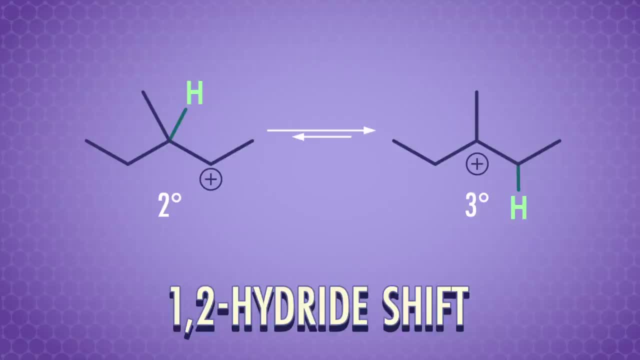 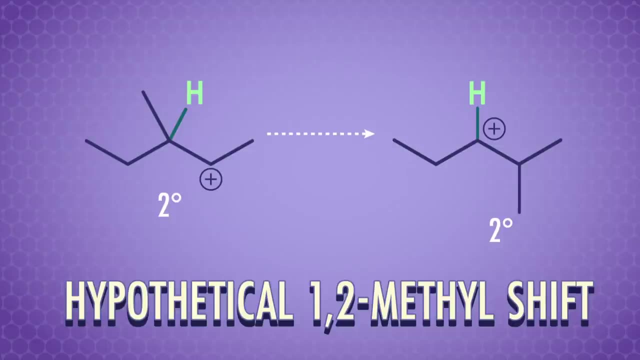 charge on the carbon it abandoned. Now there is a methyl group here too, so I guess we could try a 1,2-methyl shift again, but that actually wouldn't help us much. See, the hydride shift creates a tertiary carbocation when we had a secondary carbocation. 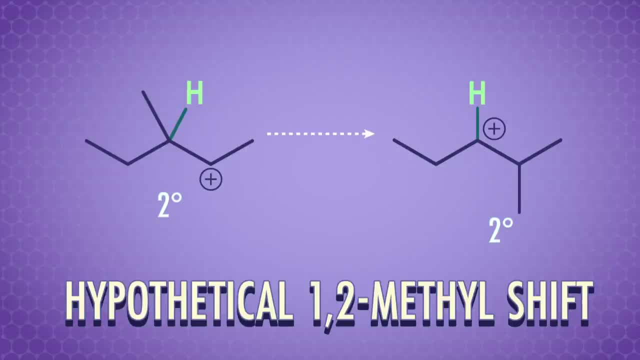 But if we were to do a methyl shift, it doesn't help with the stability. These two secondary carbocations are energetically the same, So we need to remember that. rearrangements don't just happen for the heck of it. They form a more stable intermediate. 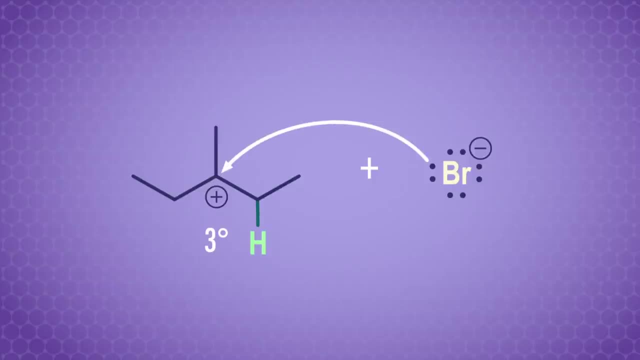 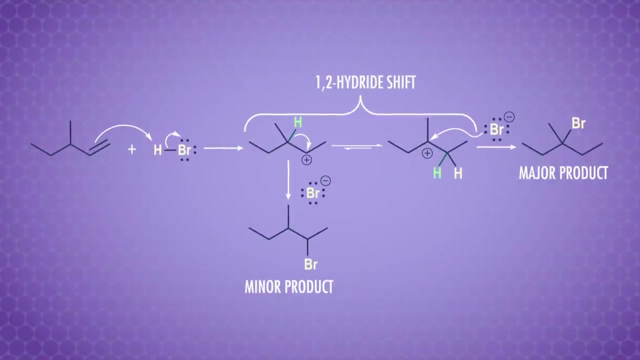 After we do the hydride shift to gain stability and the bromide does its nucleophilic attack, we get the major product that we see in the lab – 3-bromo-3-methylpentane. This is another reaction that has two possible roadmaps and a major and minor product. 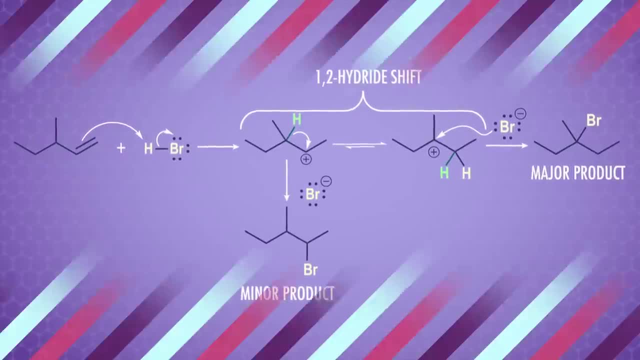 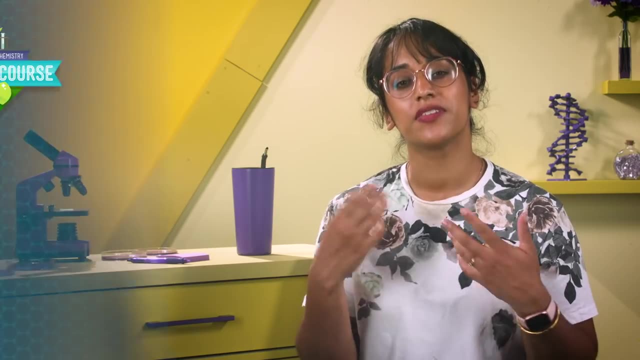 It just used a different kind of shift to help increase carbocation stability. Throughout organic chemistry, energy and stability will continue to be guiding forces as we puzzle our way through reactions, But for this episode we learned that the cis-trans nomenclature for alkenes is limited. 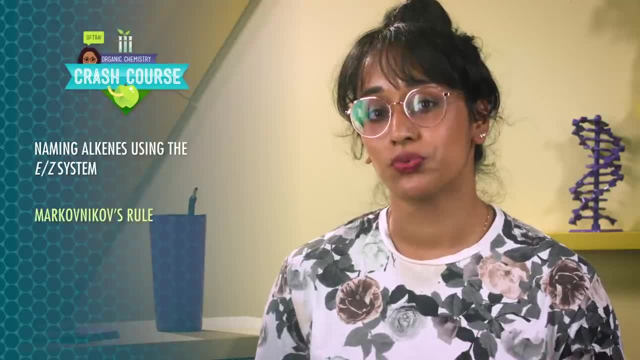 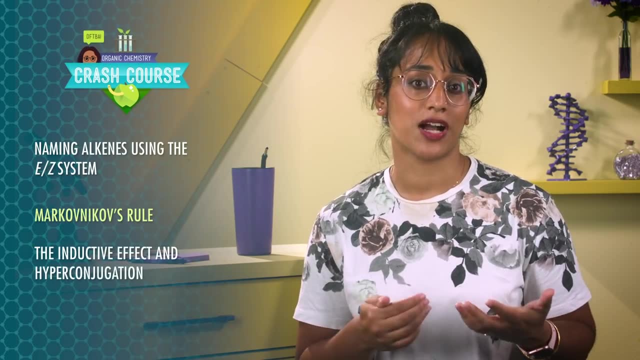 so we can use the E-Z system for more precision. Markovnikov's rule can help us predict products of addition reactions involving alkenes. Carbocations are stabilized by the inductive effect and hyperconjugation And we have to inspect alkene addition reactions for possible rearrangements through 1-2 shifts. 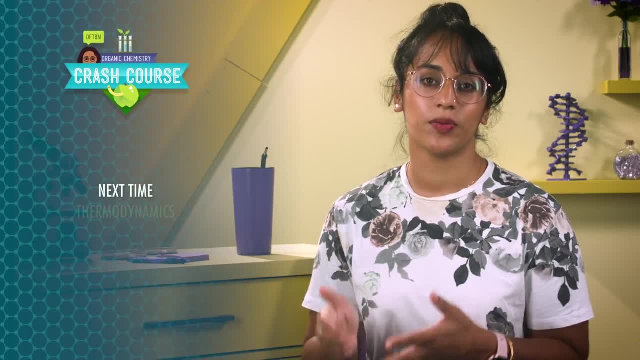 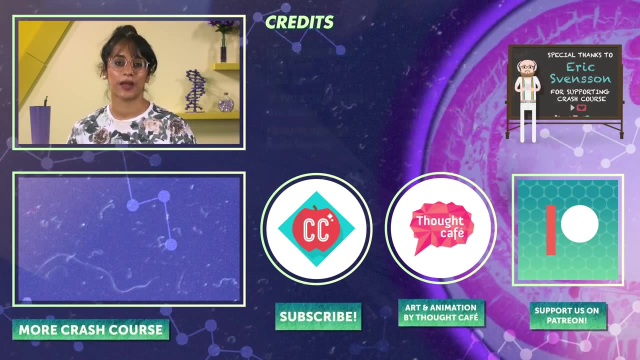 that make more stable carbocations. Next episode we'll get into thermodynamics and how to use free energy and kinetics to help us predict reaction products. Thanks for watching this episode of Crash Course Organic Chemistry. If you want to help keep all Crash Course free for everybody forever, you can join. our community on Patreon.